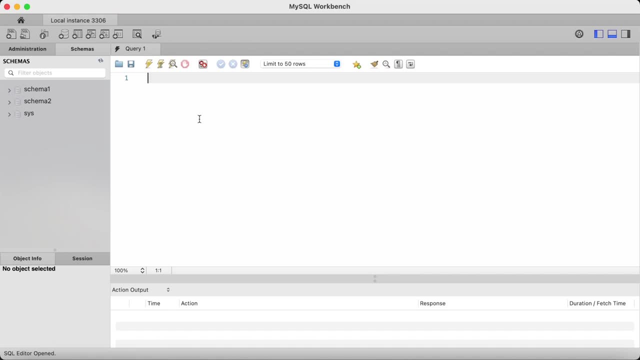 the host that this user is connected to. So for user1, it would be user1 at user1.sql. localhost. Enclose the username and host name in single quotes. In my schema- one schema- I have a table called emp, which is a table that contains fictitious. 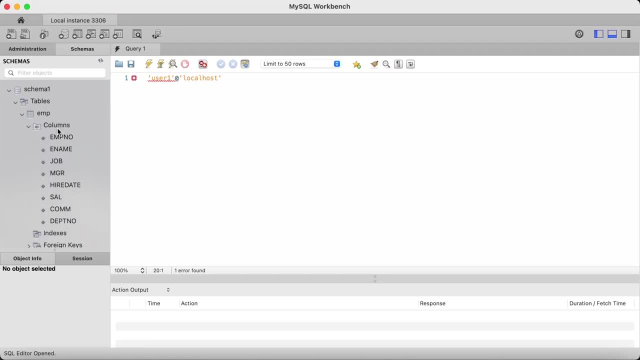 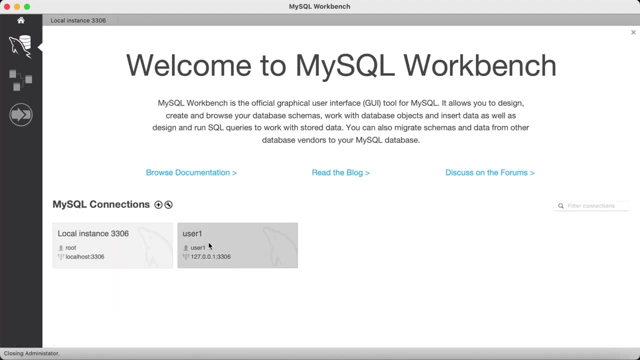 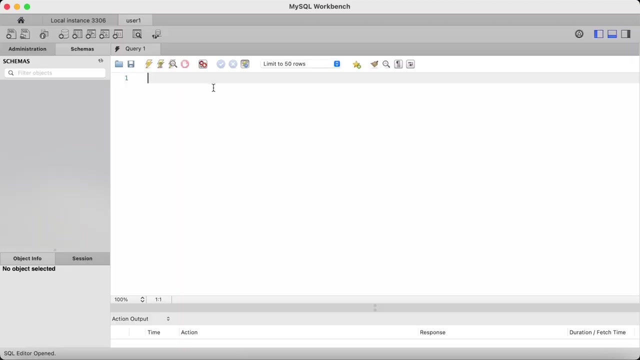 employee information. So I'm now going to access my user one account And, as you can see, at the moment I cannot see the schema or table because I don't have access to it. So I'll go back to my root account. 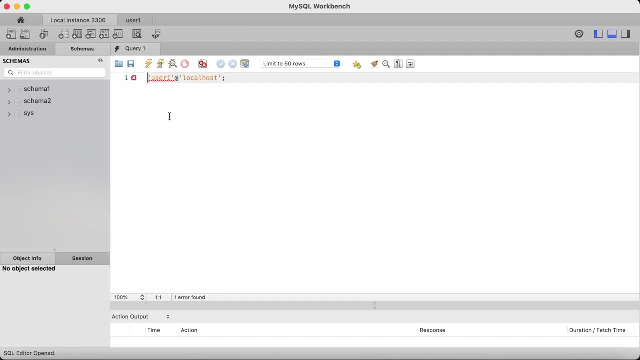 which is on this tab here and grant access to user one. So I type grant all and I type all because I'd like to grant all privileges. If I only wanted to grant, select or insert privileges, I'd type that here instead. But I'll stick. 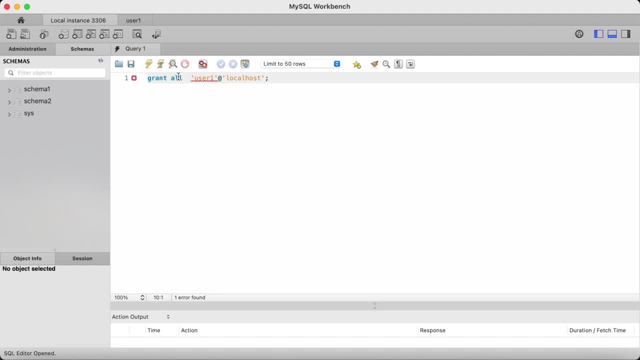 to grant all privileges for now. Grant all on the schema name, followed by the table name I would like to grant access to, which will be the emp table in schema one, And then you type to user one at localhost And, as you can see, that has been successful. 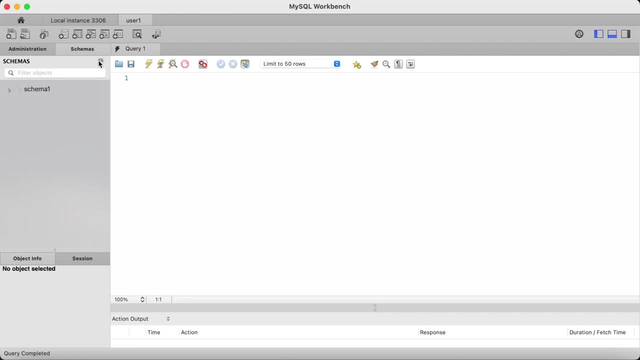 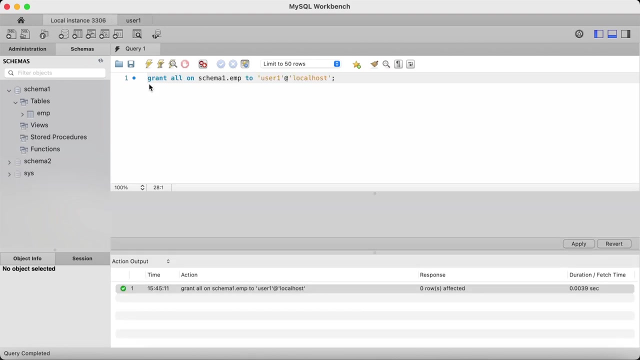 Now we'll go back to my user one account refresh and now you can see the schema and the table name. If I query the emp table, You can see that it works. I'm now going to go back to my root account and revoke access to the user one for schema.